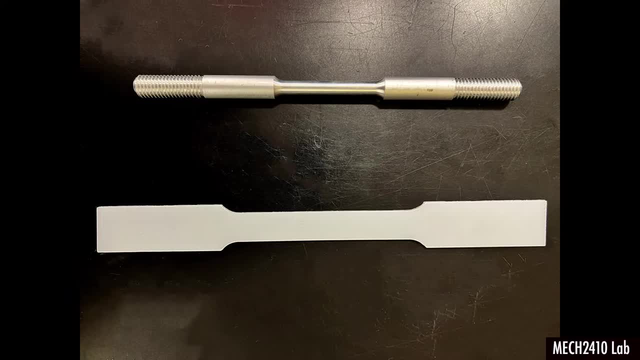 going to use for the test. The top one is the aluminum sample. It is in a cylindrical shape. The bottom one is a polymer sample. This polymer is polyethylene. It is a thin slide. First we are going to measure the gauge length of both samples. That is L0 shown. 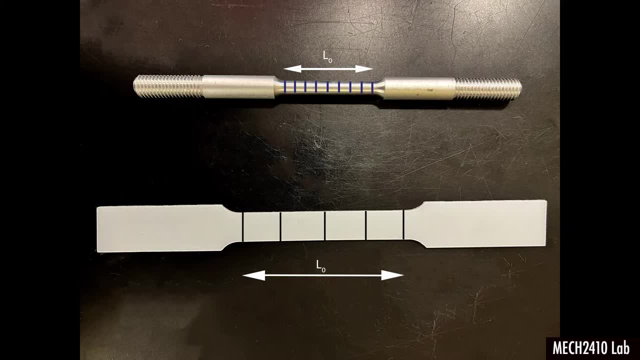 in the picture here. It is a reference length that we are going to use to measure the elongation in the tensile test. Next, we are going to measure the cross-section, The cross-sectional area for the cylindrical shape aluminum and the thin slide polymer. 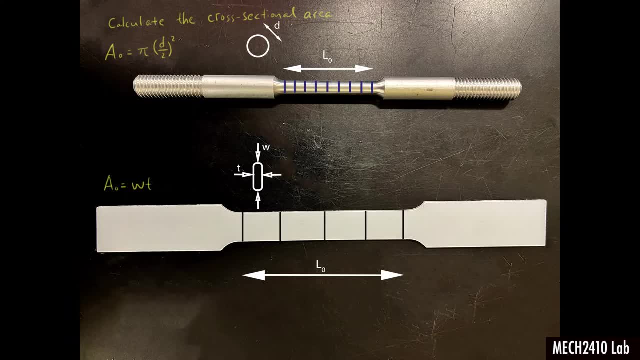 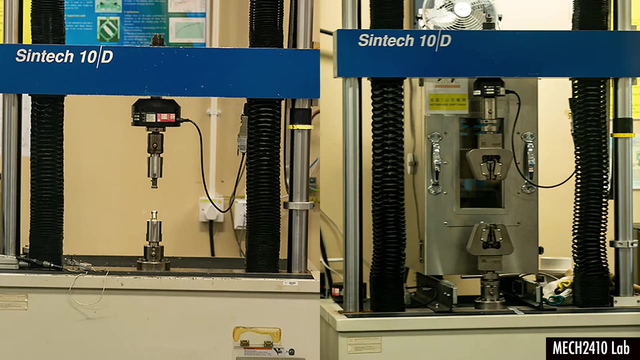 Next we are going to calculate the cross-sectional area for both samples by the formulas listed here. Then this area will be used to calculate the engineering stress for the tensile test. We use different sample grippers to mark the different types of samples. The left-hand- 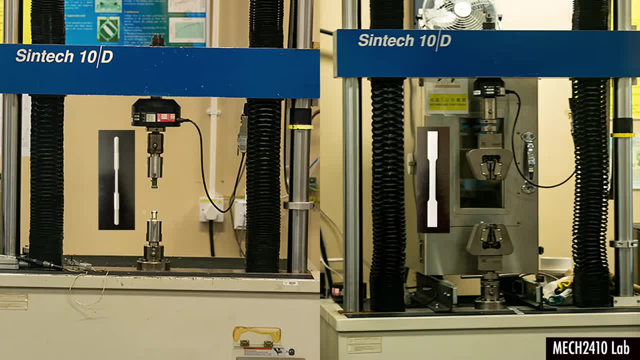 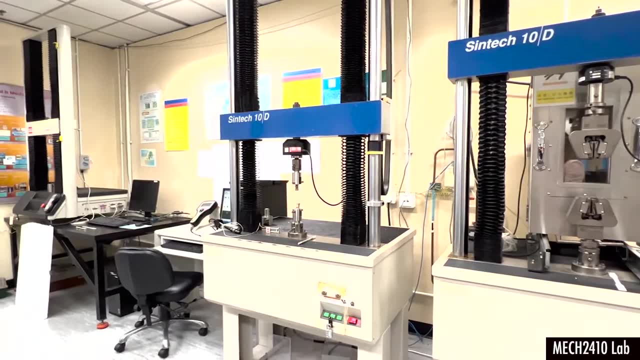 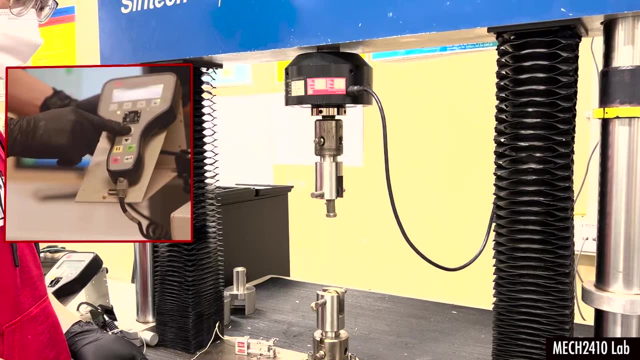 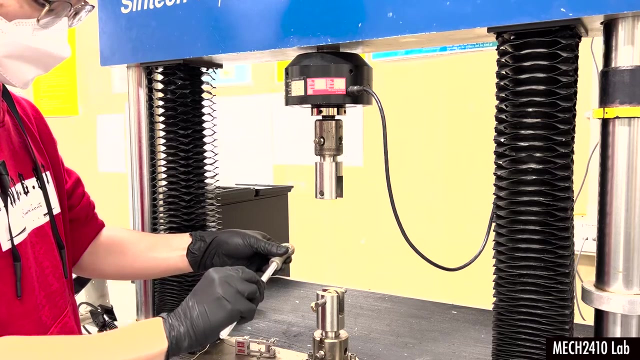 side is for aluminum, The right-hand side is for polymer. Very good, Now we have everything. We can get started our tensile test. We'll use this gripper to mark the aluminum sample. The spacing can be adjusted by the control panel. The aluminum bar is screwed tight to the gripper, as demonstrated here. 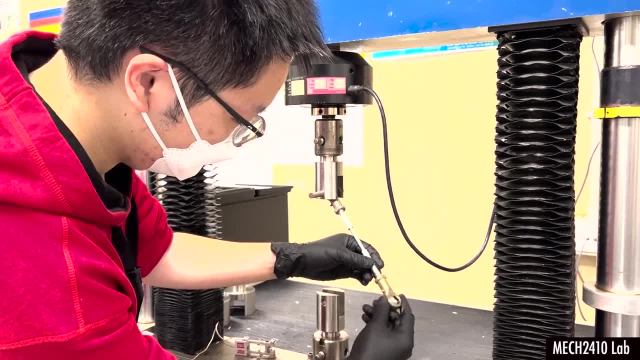 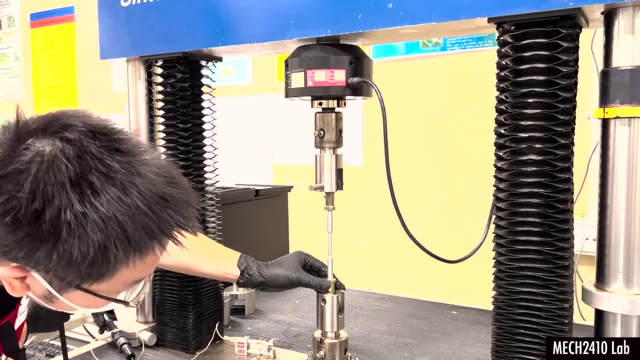 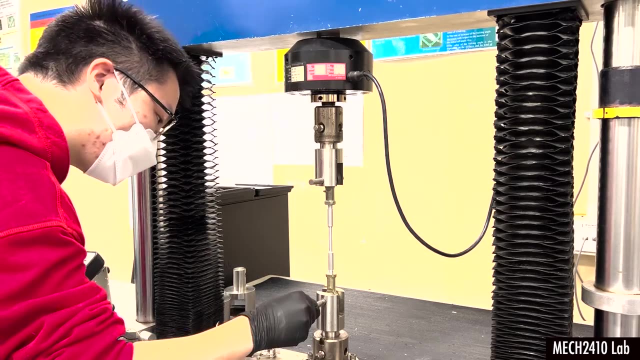 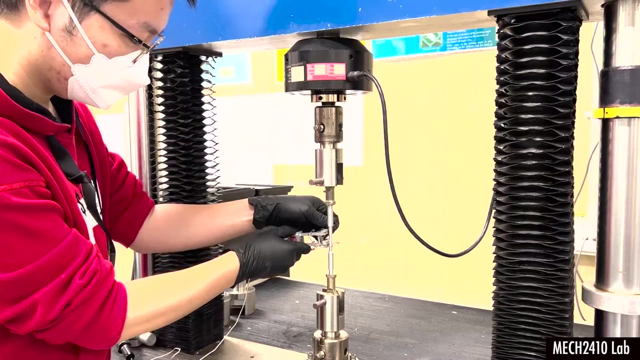 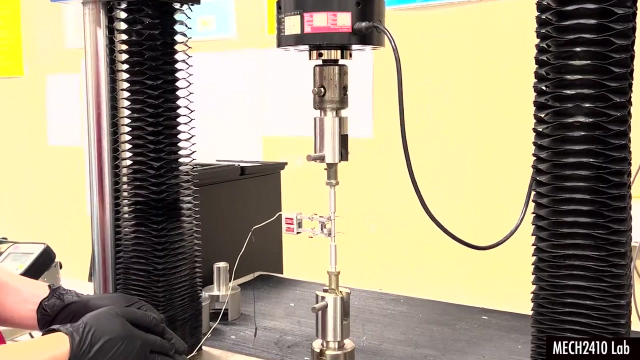 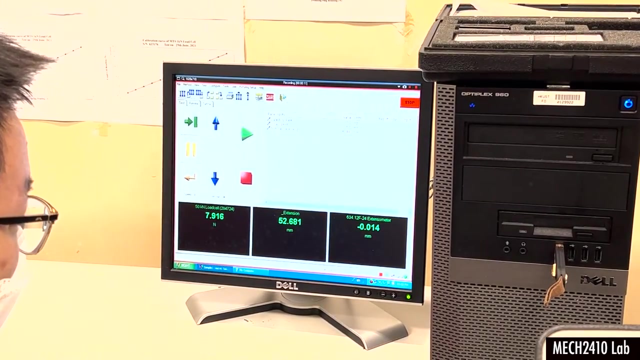 After fixing the top part to adjust the displacement, to let the bottom part of aluminum bar slide into the lower gripper and secure it. Next we insert the displacement sensor which measures the elongation of the specimen. Now we can start the measurement. 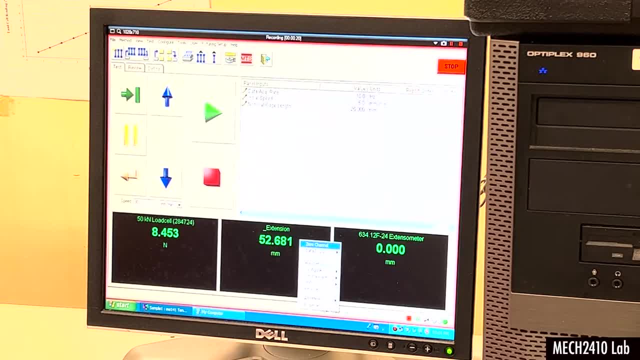 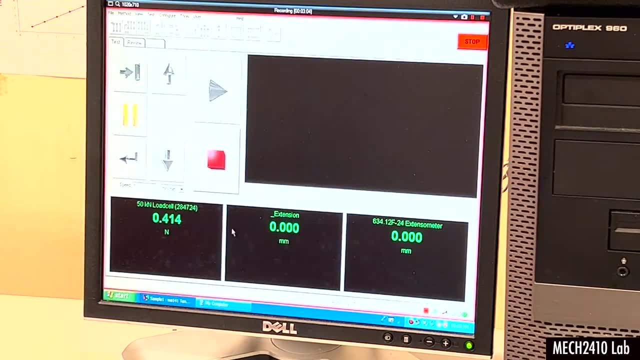 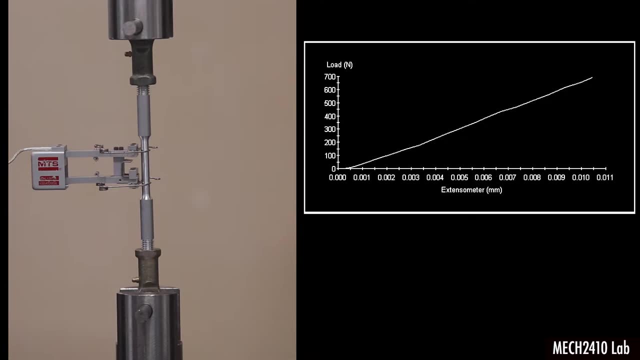 In the software window. we need to reset zeros for force and displacement. Then we can apply the tensile loads to the sample and observe the elongation. The force displacement data is recorded by the software. The aluminum specimen starts with elastic deformation. then it yields at elevated tensile. 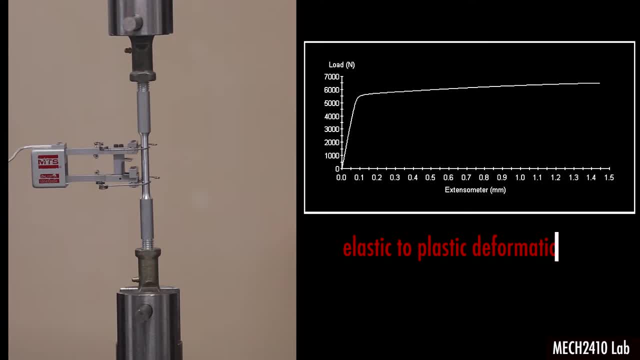 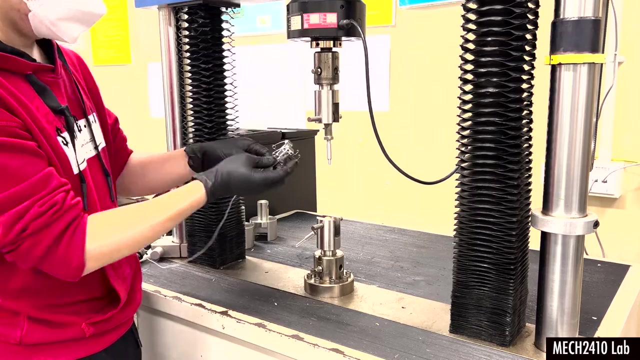 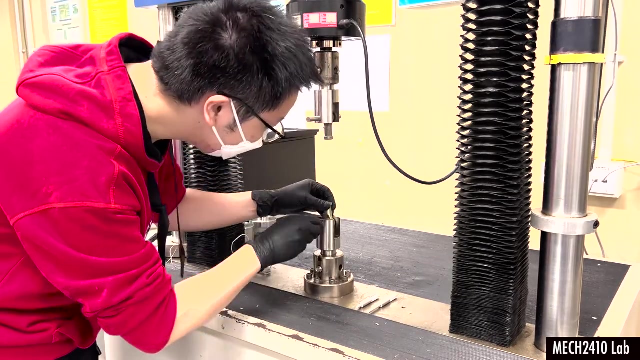 force Experience the elastic to plastic deformation. When the force level drops, it corresponds to the necking phenomenon of the cross-sectional area of the bar And finally, the material is fractured. Finally, we remove the broken specimen from the gripper to wrap up the experiment. 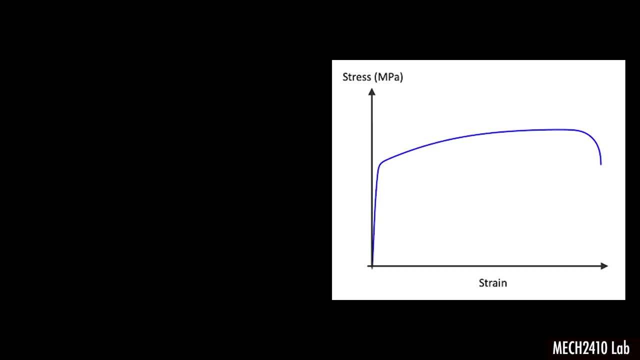 We present data as a stress and strain curve. The stress is in MPa unit and it is calculated as force per unit cross-sectional area. Strain is in MPa. Strain is in MPa. This is the elastic region. The mass is computed as relative elongation with respect to L0.. 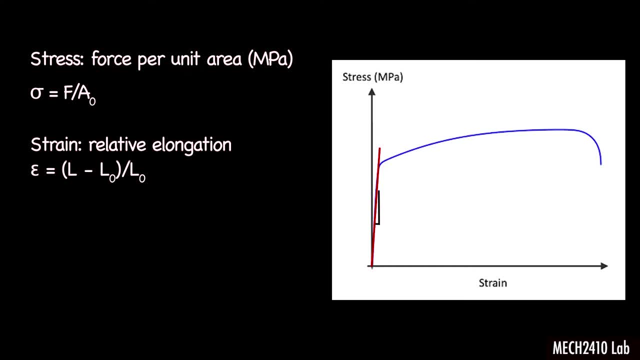 Its slope determines Young's modulus of the specimen. This is the yielding point beyond which the material starts the plastic deformation. The maximum stress achieved before fracture is usually defined as the ultimate strength of the material It's left now. It indicates how strong the material is. Now let's move on to the tensile test for polymer thin slides. 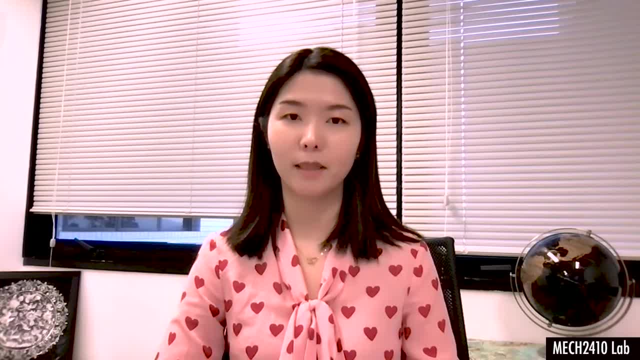 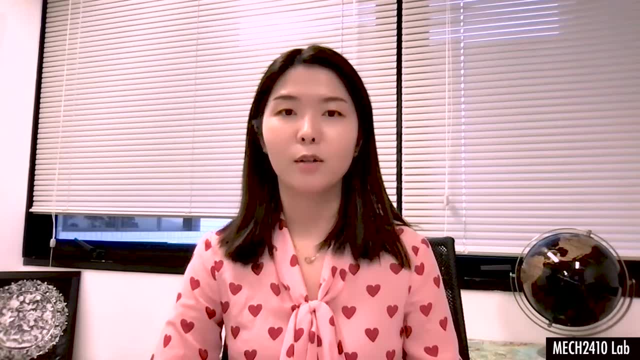 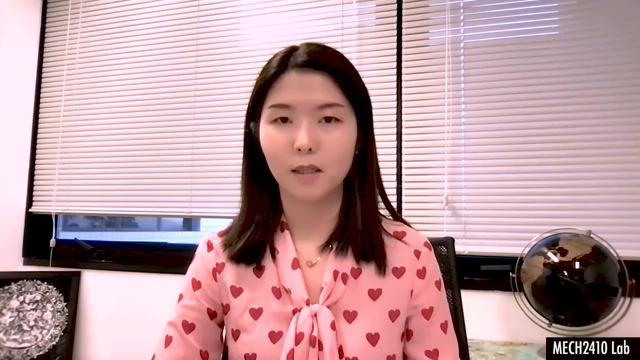 The tensile test of polymer is similar to the aluminum, except we use a different gripper. We still begin with the calibration and set force and displacement to be zero value, and then we start our tensile load and record the force displacement data And we observe similar things.